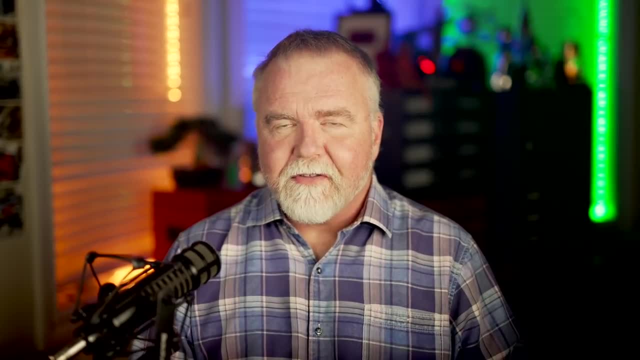 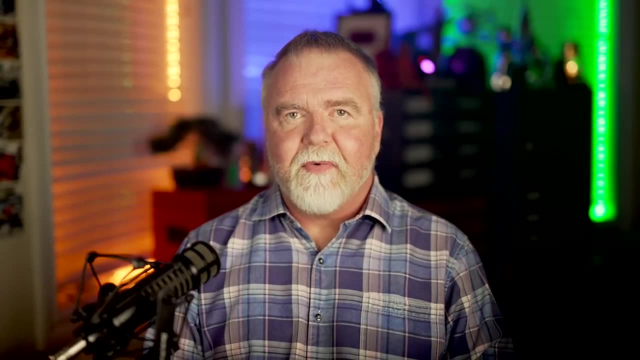 will be new and useful, so stay tuned. I think pointers are scary for everyone when you first get introduced to them. This is especially true if you're coming to C from a language like Java or Python, where they're not something that you commonly see, Just when 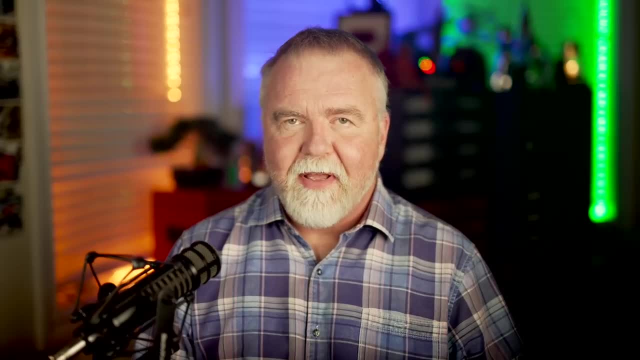 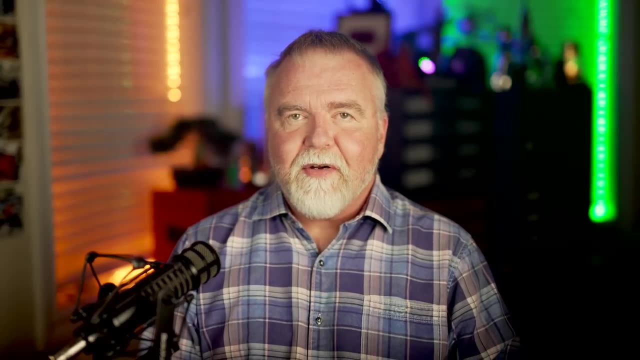 you think you've got programming sorted out, you make the jump to C and it's just a mess of pointers and punctuation. Well, rest assured, pointers are only scary because they look that way. They're actually an incredibly simple concept once you understand them. And today, 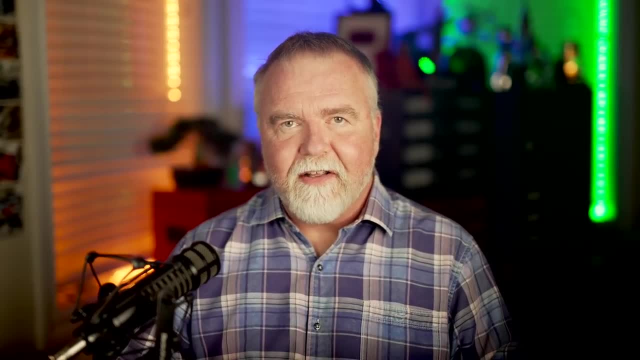 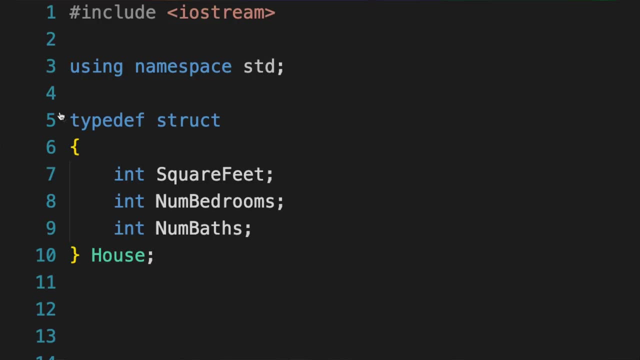 I'm going to try and get you over that hump. Let's get started. Let's consider the analogy of a house. Perhaps in C we can define a house like this as a structure that keeps track of the number of square feet the house has, the number of bedrooms. 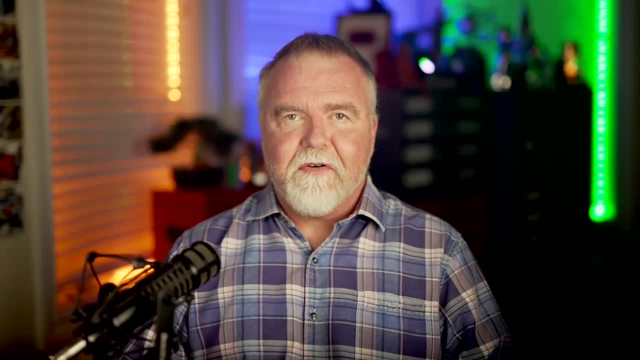 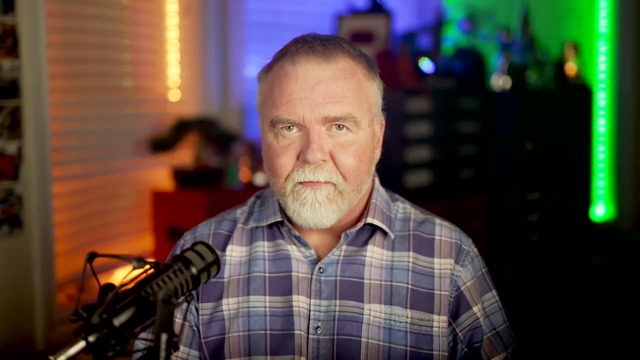 and the number of bathrooms. We create a house object in our code, whether it's a global variable or just a local one, and, as you're likely aware, the house object is stored somewhere in the computer's memory And all the memory in your computer is numbered with an address from byte. 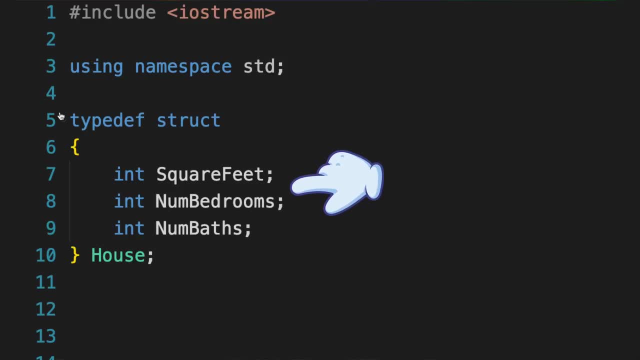 zero on up to the top of memory. Our house object has three integer values, so it's going to be 12 bytes of storage in total. The compiler finds a place for it and puts it there, and that's all there is to it. Now. we normally 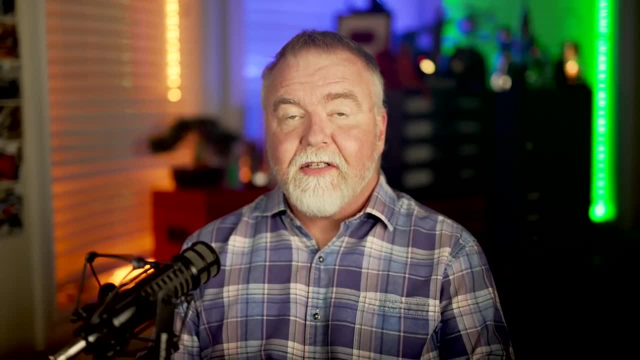 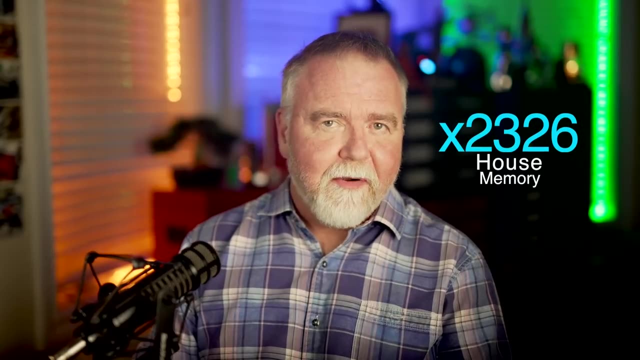 have no idea where, in memory, our house is going to be stored, but let's say, in this case it gets placed at address 2326.. Now what if you want to tell someone that there's a party at this house? How would you go about it? Well, you could drive to the house all the way across town and show each. 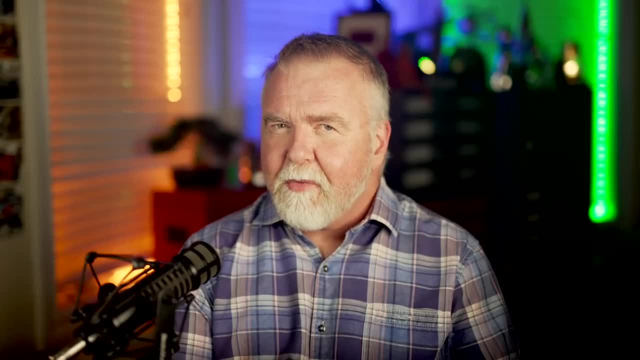 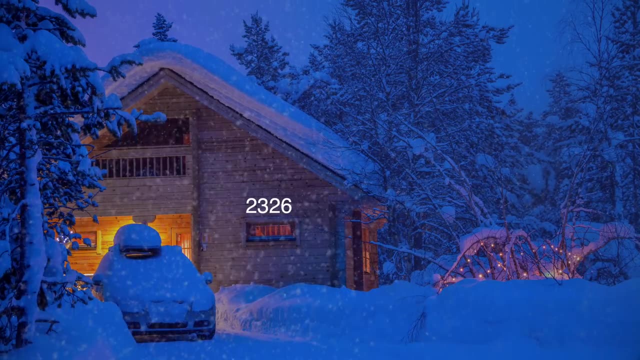 person that's being invited, which house it is and where it is. But you wouldn't likely do that, would you? What would you do? Well, you'd give them the address. You'd say: hey, the street address is 2326,, stop by and BYOB. That's way easier than taking everyone there in advance to show them. 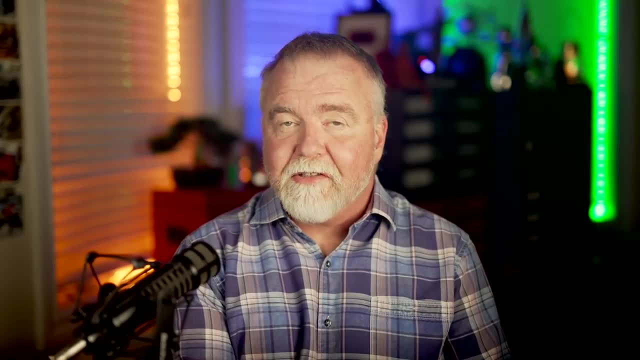 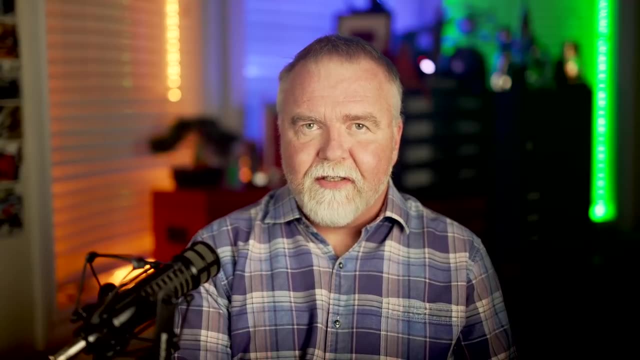 or worse, creating an entire copy of the house to demonstrate what it looks like so they can recognize it. And at its core, that's all that. a pointer is a variable that holds the address of some object. It's just the memory address of something interesting, like a house, Or in C. 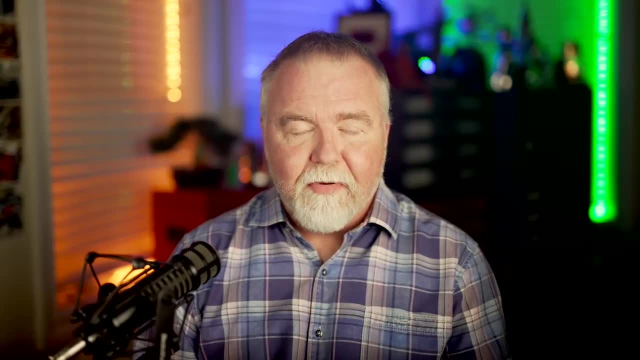 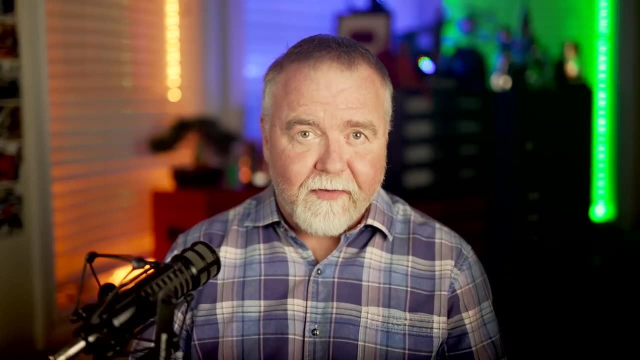 it might be a structure or a string, or even a simple integer, But if you create a pointer to something, all you're doing is storing its memory address in a variable that we call a pointer. What makes pointers powerful is that you can access and use the object that's being pointed. 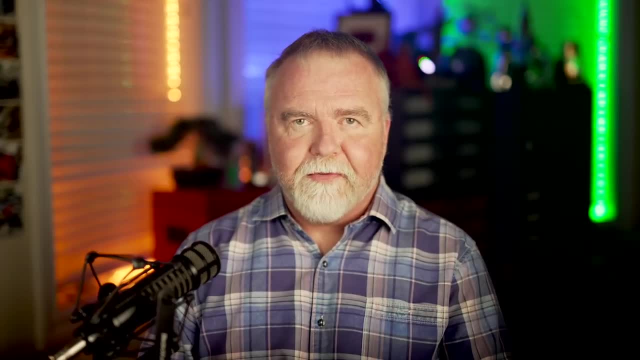 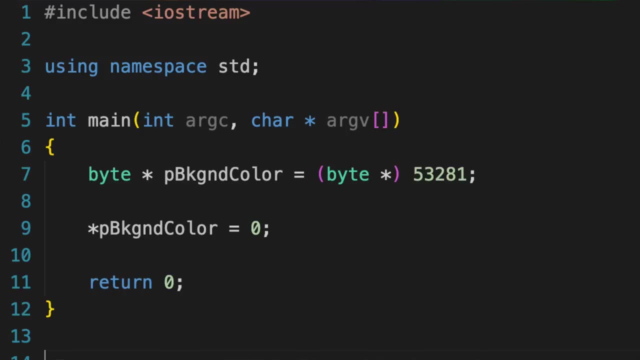 to by the pointer. You don't need a whole copy of the house object, You just need to know its address. Let's look at an example so simple that it's painful. On the Commodore 64, you can change the background color of the screen by changing the byte and memory at address 53281.. If you set 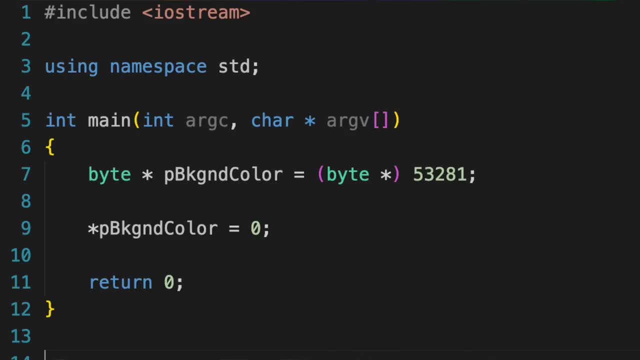 it to zero, the screen will turn black. Now how would you do that in C? Well, we know two things: We know the type, which is a byte, and its address, Which is 53281.. So we create a byte pointer called pBackgroundColor and set it to point. 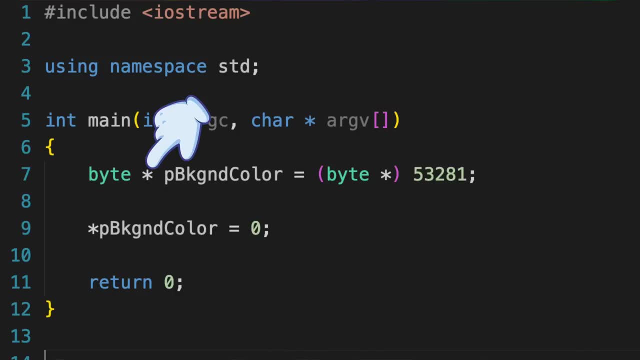 to address 53281.. In C, when we're creating a pointer, we add a star in front of the variable name to indicate that it's a pointer. So for a pointer to a byte in memory, we declare it as byte star: pBackgroundColor. Syntactically that means that pBackgroundColor is a pointer to a. 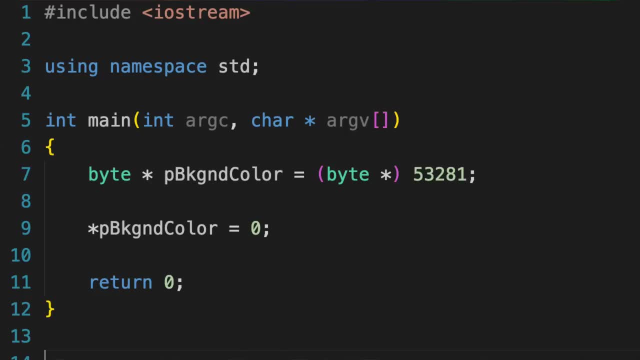 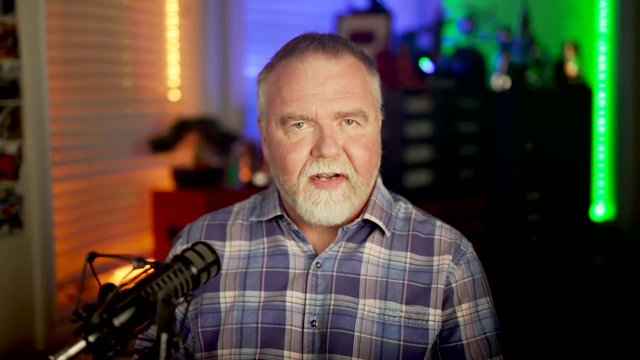 byte in memory. It's a variable that will hold the address of a byte. So pBackgroundColor is a pointer and it points to address 53281.. But now, how do we change the contents of that address? Well, in C we use the star operator again, Putting a star in front of the variable name. 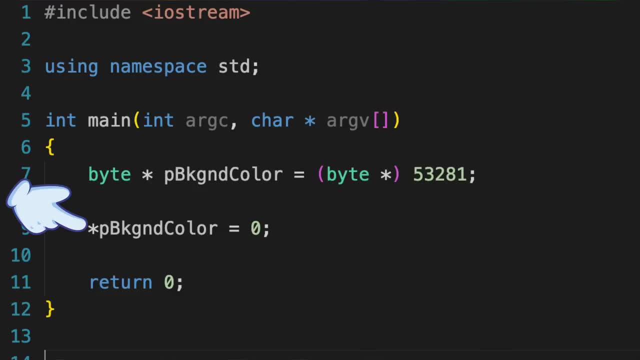 when you're using it means that you're referring to the thing being pointed at, Or, put another way, at the contents pointed to by the pointer. In this case it's a byte, so star pBackgroundColor means the contents of memory location 53281.. When we store a zero at that location, 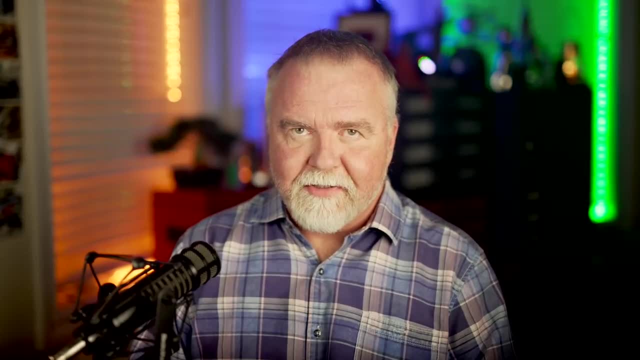 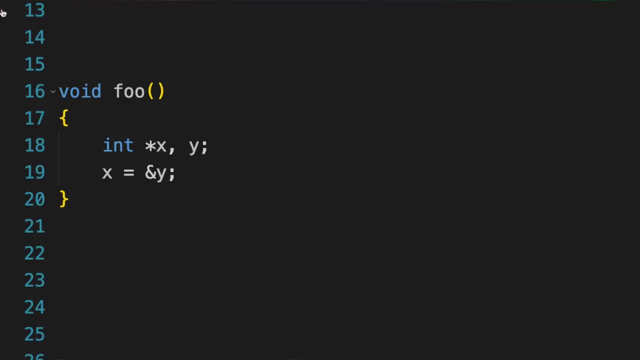 the screen will turn black. One little syntactic caveat here is that we don't want to use a pointer for any of these declarations. The star must proceed. each variable name that you're declaring as a pointer. It decorates the variable, not the type. 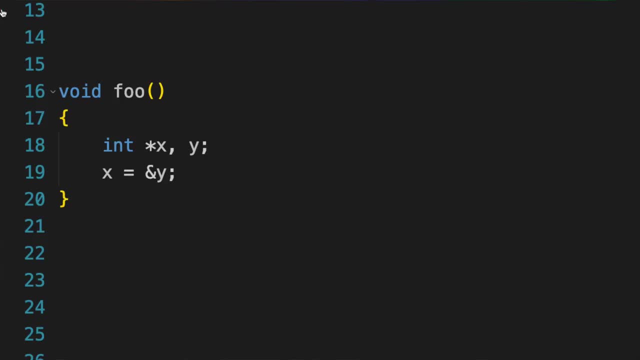 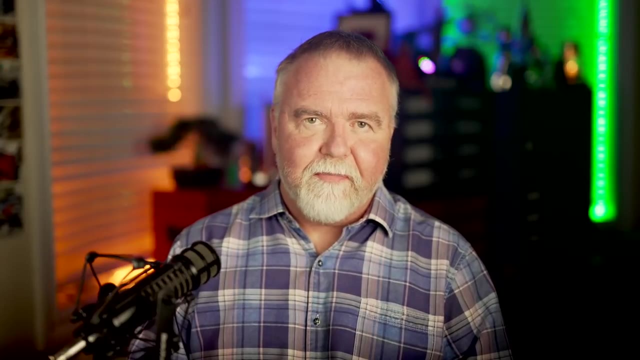 name. So if you were to write int star x, comma y, you're declaring one pointer to an integer and one actual integer. If you wanted two pointers, both would have to have the star. Pointers to bytes and integers are all well and good, but what about pointers to more complicated things? 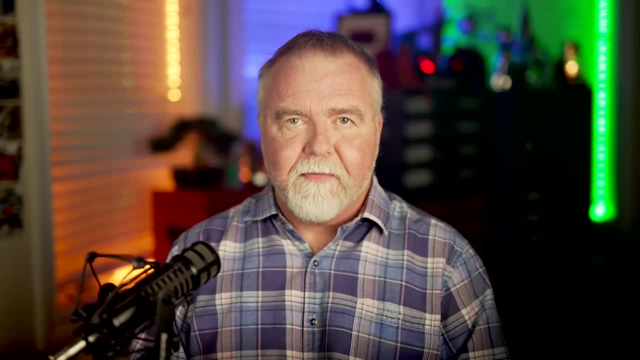 like objects. Well, let's create a house using our house class, the one that includes the square footage, the bedrooms and the bathrooms. We'll give it the same specs as the house I grew up in. but we'll give it the same specs as the house I grew up in, but we'll give it the same specs as the house I grew up in. 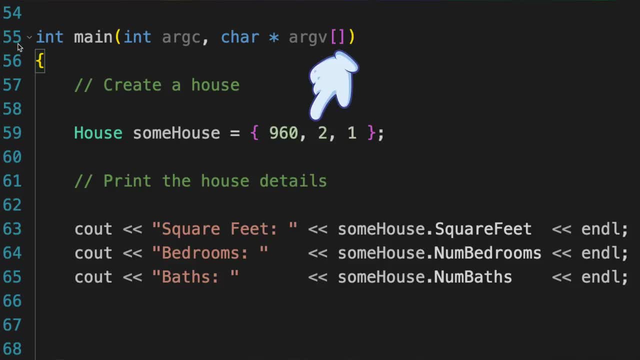 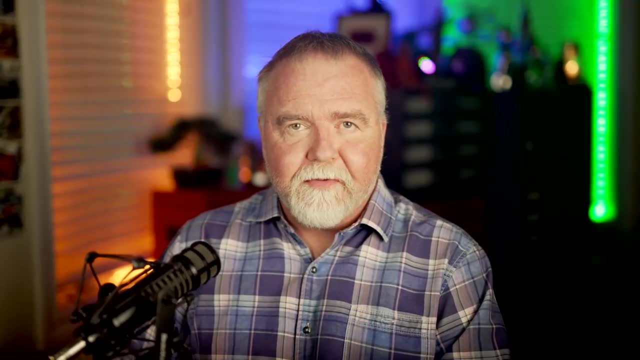 but we'll give it the same specs as the house. I grew up in: 960 square feet, two bedrooms, one bathroom, and dad got first dibs on the bathroom. If we want to print out information about the members of the house structure, like the number of bedrooms, we use the dot operator. 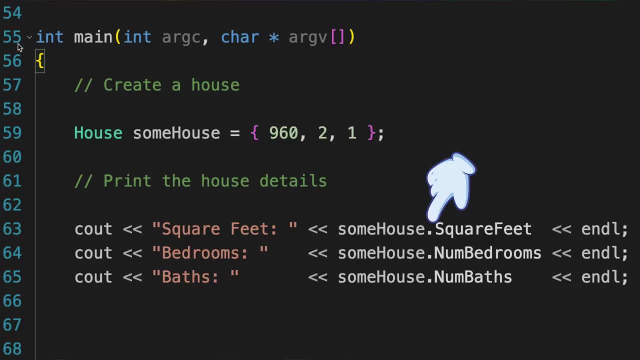 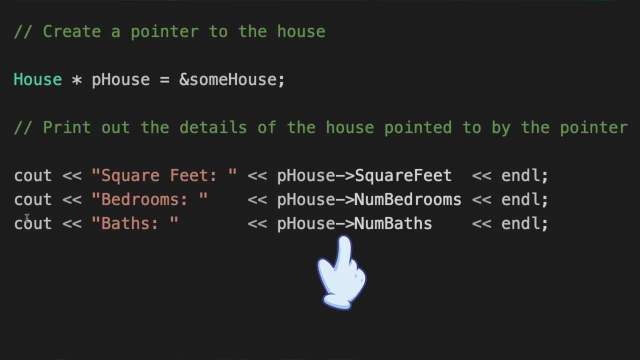 The dot operator indicates you're looking for a member variable of the class. The only difference when using a pointer is that you use the arrow operator on the pointer instead of the dot operator on the object. The arrow means go to the object being pointed to and then get this member variable by its name. The arrow is the same. 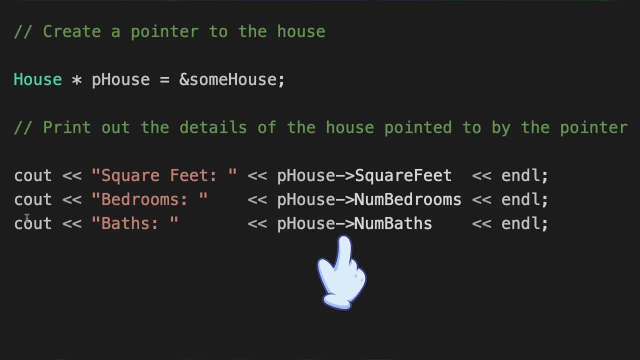 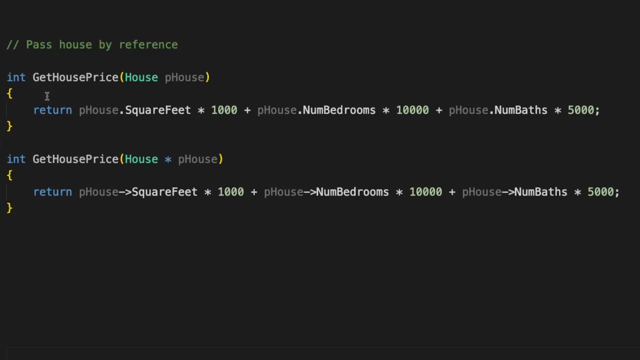 as a dot, but it indicates you're using a pointer to the object and not just the object itself. Here we have two versions of the getHousePrice function. Both price the house in the exact same way, but the first version accepts an actual house object as an argument When a caller calls this. 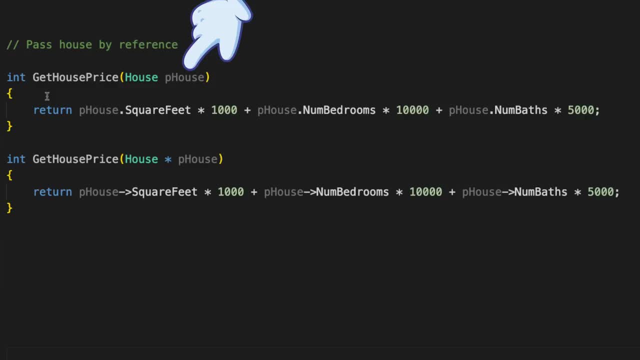 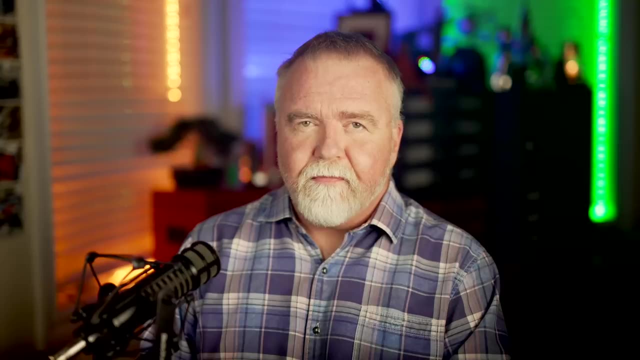 function. the house object they provide will be copied and used as the argument within this function. Depending on the size and complexity of the house structure, that could be an expensive and wasteful operation. Why is it wasteful? Well, because, just like in real life, there's no reason. 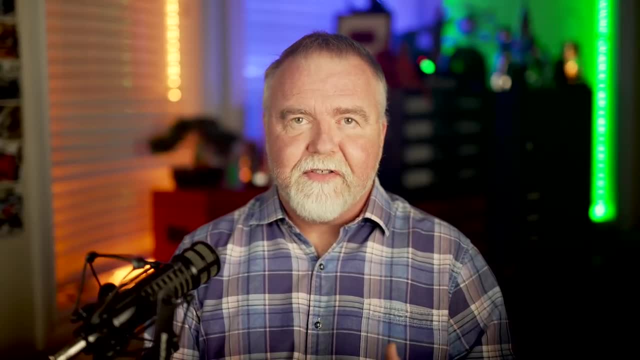 to bring your house to the house structure. It's just a wasteful operation. Why is it wasteful? Well, because, just like in real life, there's no reason to bring your house to the appraiser for an appraisal. The appraiser comes to you based on the address of the house, And that's what our second version. 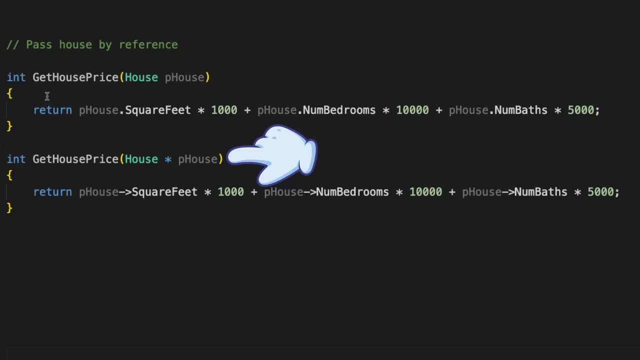 of the function does. It accepts a pointer to the house or the house's address, and then uses the arrow operator in exactly the same way as the first function used the dot operator. The difference is that the second version is using a pointer. It indirects through 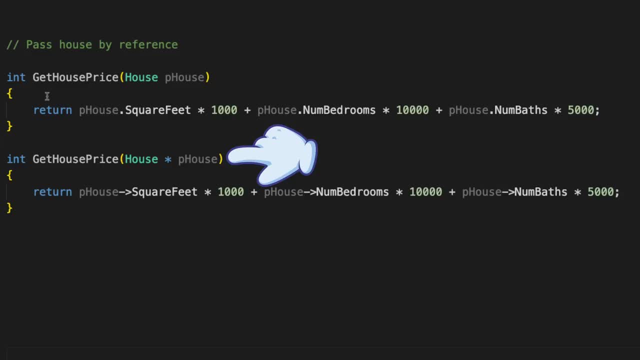 the pointer and looks up the members of the object that it's pointed to. Another way to look at it is that the first version of the function accepts an argument in a pass-by-value manner and the second version is a pass-by-reference. Pass-by-value means that the object is passed as a complete. 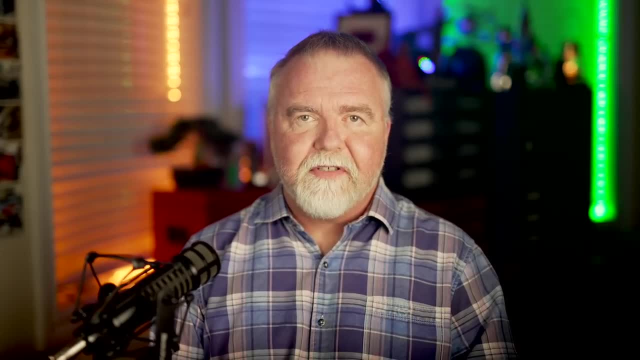 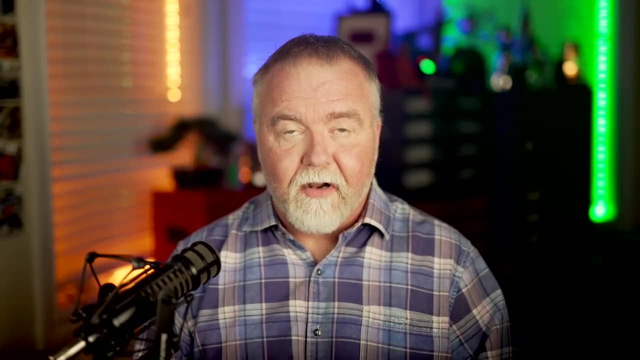 copy. Pass-by-reference means you're just passing the address of the object in the form of a pointer. Pass-by-reference is usually far faster and more efficient than pass-by-value, at least for larger types. On a 32-bit system, a pointer is 4 bytes, and so that's all that's. 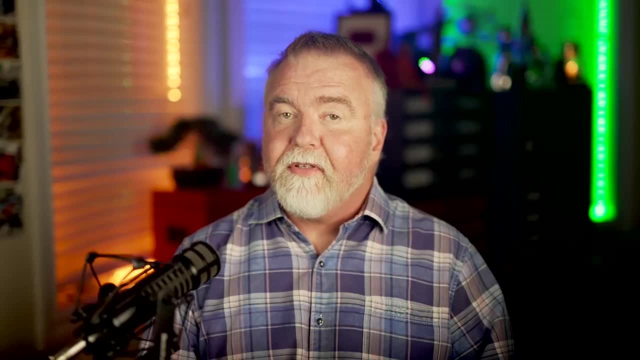 passed through the function, no matter how big or complicated the object being pointed to is. Now that you hopefully have a basic grasp of what a pointer is, we can talk about some important concepts related to pointers. Let's take a look at a pointer. 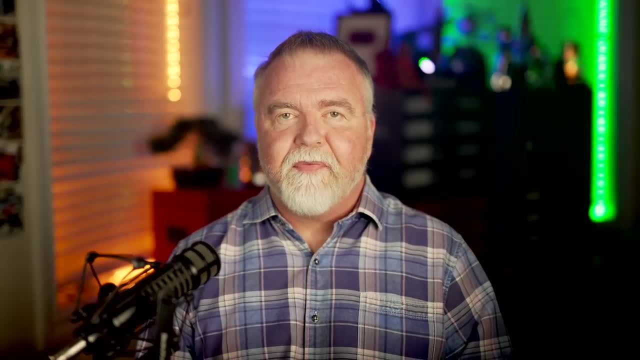 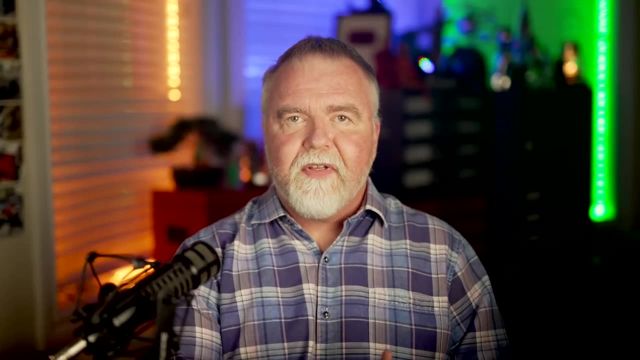 The first we've already seen, and that is the concept of indirection. The main thing to remember about pointers is that they do not hold any actual values or types, but instead hold the address of those values. In other words, they point to the location of memory. 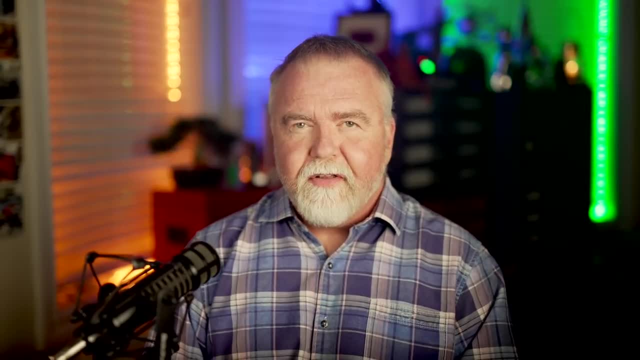 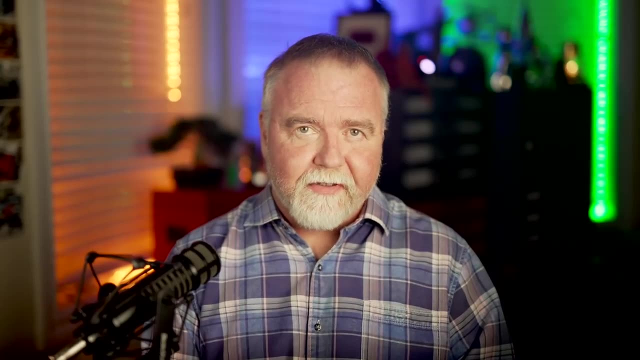 where the values are stored, and hence the name pointer. This level of indirection is often the most difficult concept for new programmers to grasp. Another important distinction is between arrays and pointers. It's common for beginners to be confused between pointers and arrays, as they 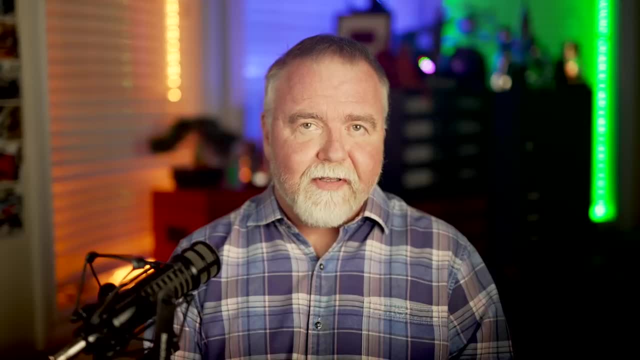 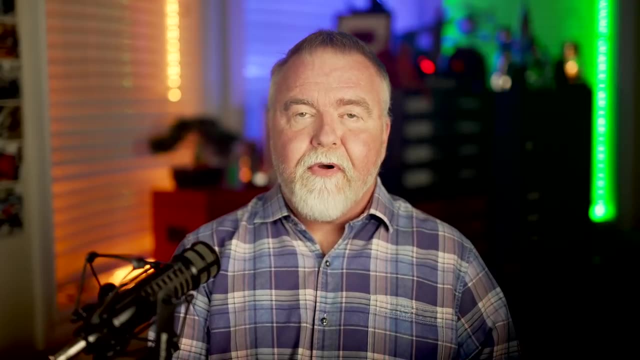 sometimes can be confused by the name of the pointer and sometimes by the name of the object. However, they are fundamentally different. An array is a contiguous chunk of memory holding multiple values of the same type, like a character string. A pointer, on the other hand, is a variable. 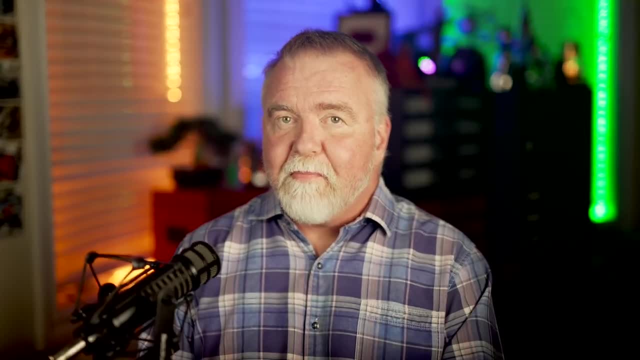 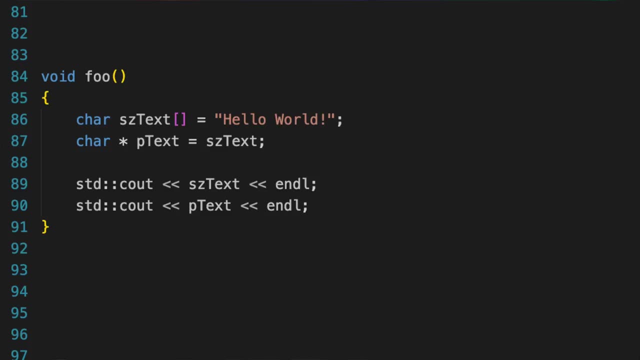 that holds the address of the first value. The big lightbulb moment often happens when one finally understands that when an array is used as a pointer, it decays into a pointer to its first element. After all, if your pointer points to the first element of an array of objects in memory 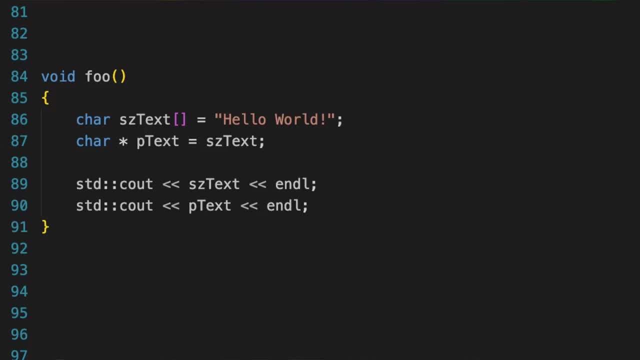 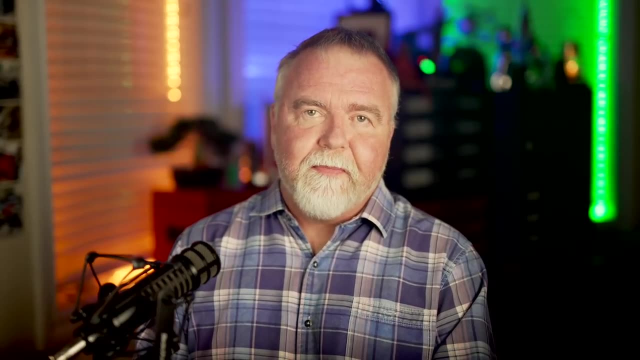 as long as you know how many elements there are and where they start. using a pointer to an array is largely the same as using the array itself. Pointer arithmetic is another complex aspect to grasp, mainly because it involves manipulating memory. addresses directly The big moment of 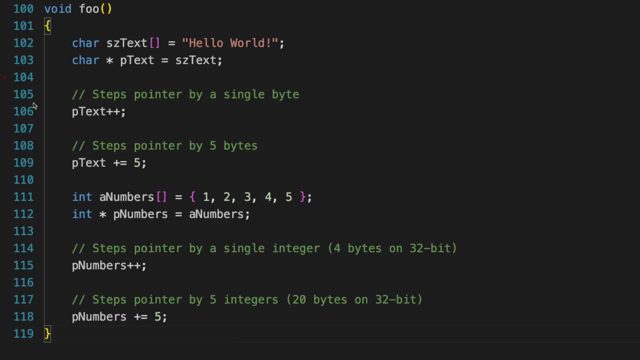 realization here often happens when you realize that adding or subtracting from a pointer value actually moves it by a multiple of the size of the type that it points to, not by just one byte. Now, if you've got a pointer to a character string in memory, every time you increment the pointer. 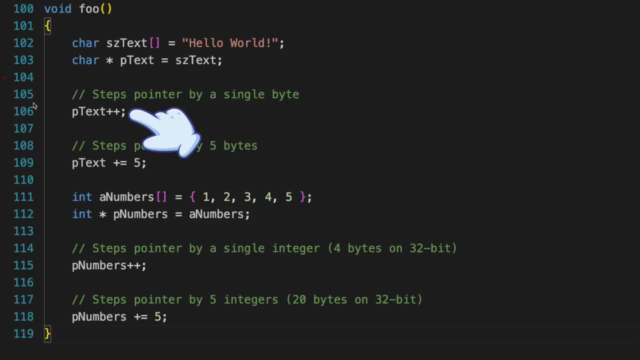 the address it contains will step forward one byte, because each character is one byte. If you've got a pointer to 32-bit integers, however, every time you increment the pointer or add one to it, the pointer will step ahead by four bytes, because that's the size of the 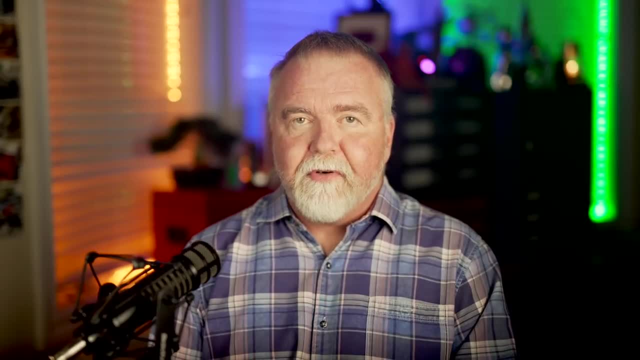 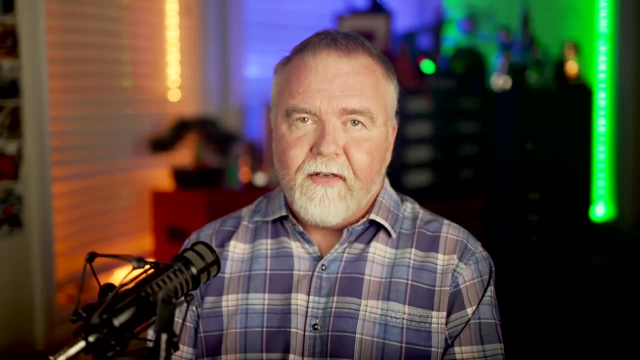 objects that are being pointed to. And so if you had a pointer to an array of house objects, every time you incremented the pointer it would step by 12 bytes, since that's the size of the structure. Likely the most common pointer you'll run into is the character pointer. A character pointer. 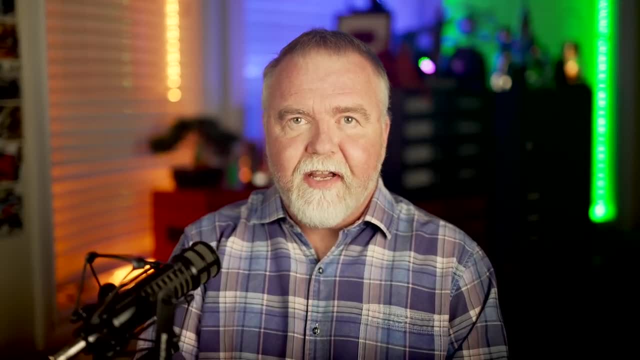 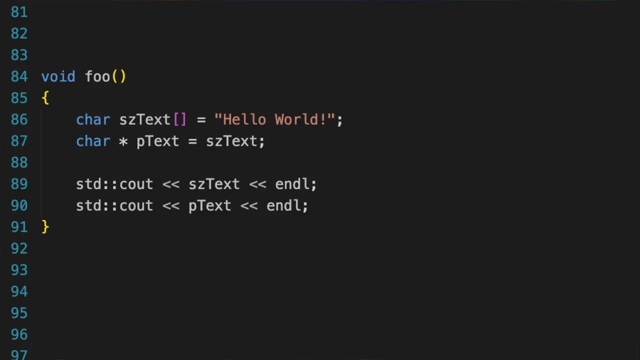 or sometimes called char pointer contains the address of the first byte of a string in memory. In C, strings are terminated at the end by a zero byte. You can almost treat a character pointer and an array of characters as being the same thing, and most of the time you'll be right. 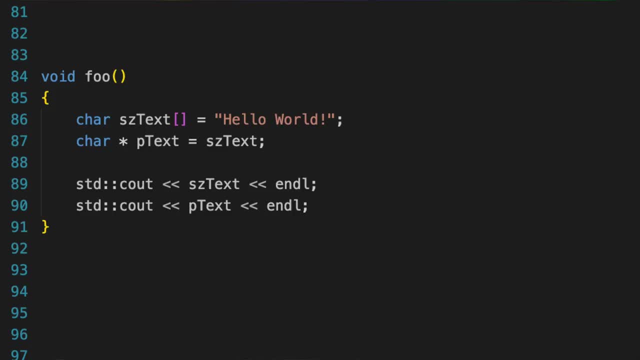 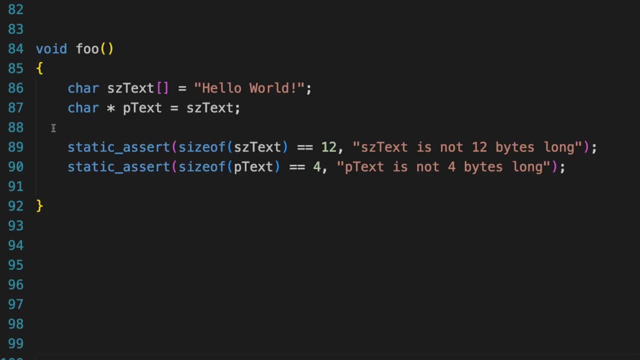 The primary difference is that a pointer is a variable that contains the address, whereas an array is syntactic sugar for the actual memory address. Furthermore, the size of an array is its actual size, the memory bytes that it takes up, whereas the size of the pointer will just be 32 or 64 bits, depending on your system. 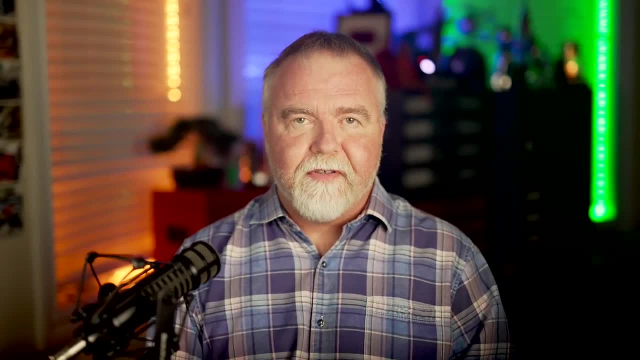 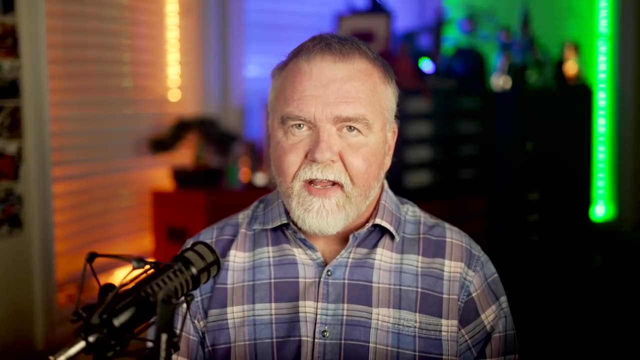 Among the more esoteric features that you might encounter are pointers to pointers. Pointers can point to other pointers, leading to multiple levels of indirection. This concept is a bit tough to understand, but it's crucial when dealing with dynamic data structures like trees and graphs. As perhaps the simplest example of a pointer to 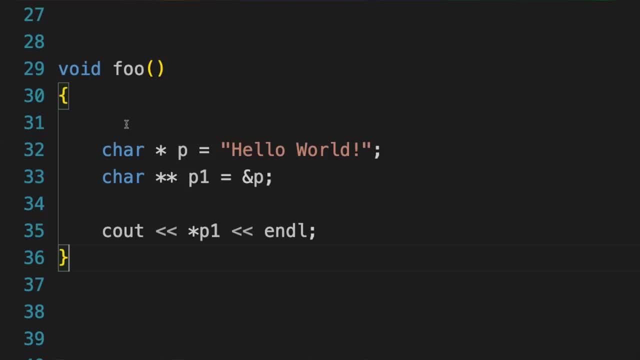 a pointer. let's imagine that we have a character string and a pointer called p, which points to the first byte of it. We then create a pointer to a pointer indicated by the two stars and set it to the address of the first pointer. So at this point, p points to the string itself. 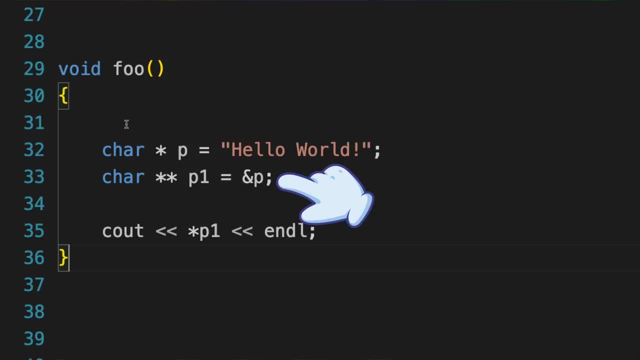 and p1 points to p. That means if we indirect from p1 by using the star operator in front of it we get that original pointer. We can output that to the console just like any other pointer to a string, because the contents of a pointer to a pointer is just that pointer to the string. 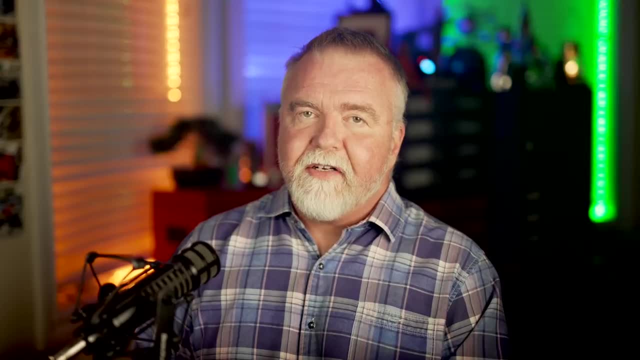 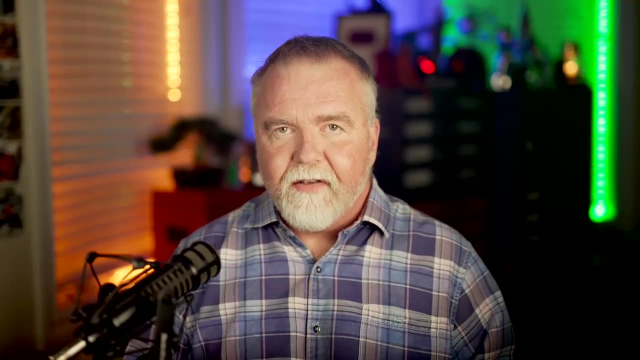 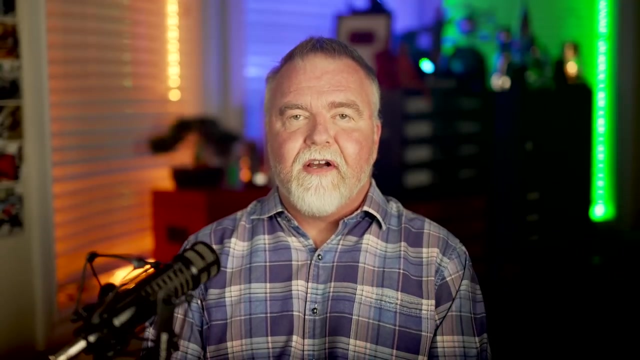 The other thing you should be aware of is the difference between a null pointer and an uninitialized pointer. Understanding that an uninitialized pointer and a null pointer are not the same can be a significant point of understanding. An uninitialized pointer has an indeterminate or random value, whereas a null pointer is a pointer that does not point to any object or function. 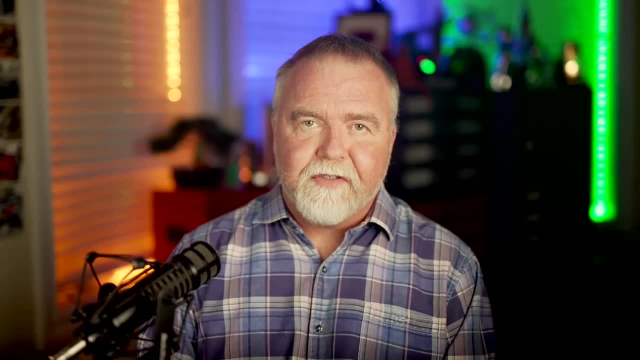 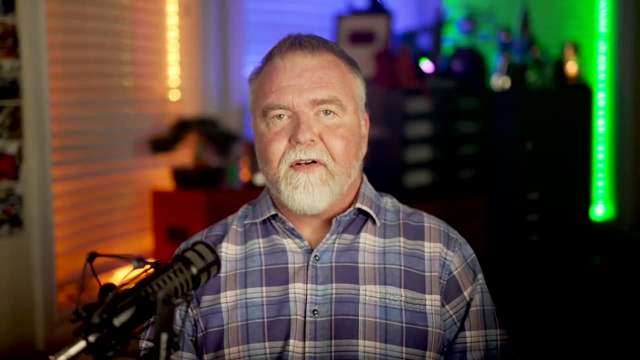 In C, a null pointer is set to zero, but an uninitialized pointer just randomly points and is useless until it's initialized with the address of a real object. Once you start working with pointers, particularly if you do any memory allocation and management, you will undoubtedly run into the concept of the void pointer. 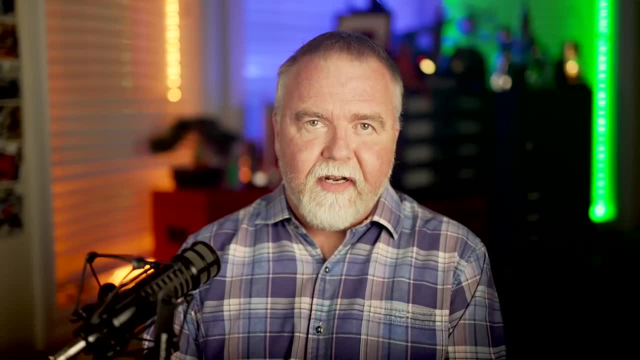 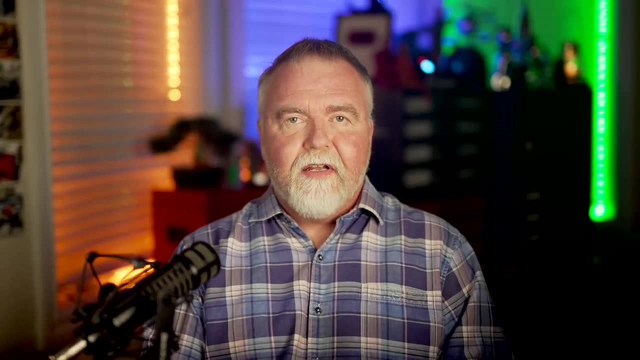 A void pointer points to an address in memory, like any other pointer, but it has no notion of what lives there. It could be a house, it could be an integer, it could be a string, It doesn't matter, It's just the address. A void pointer just points to the address and has to be. 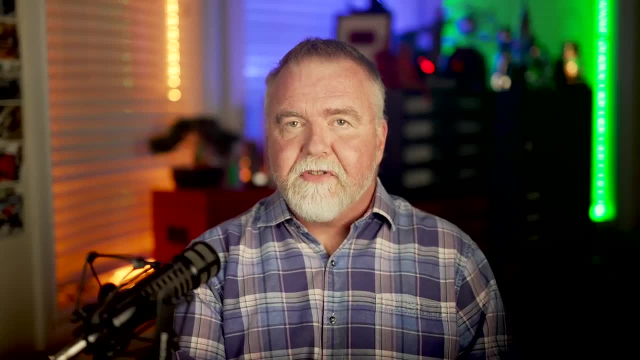 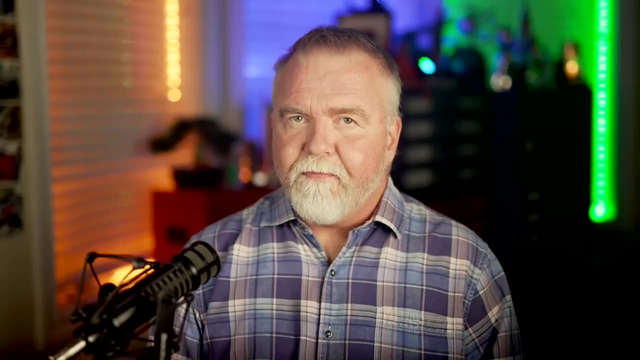 converted or cast to an object pointer before you can really use it for anything. The void pointer simply stores the memory address with no type information. Why would such a thing exist? Well, imagine you're writing the malloc API that allocates and returns a block of memory. 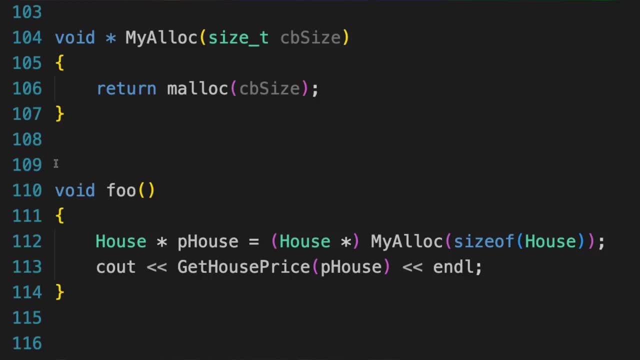 As the API writer, you have no idea what kind of object the user will ultimately place there in memory. You're simply asked for a block of memory of so many bytes and you return the address of it, and so you return it as a void pointer, not knowing what it is. The caller is then free. 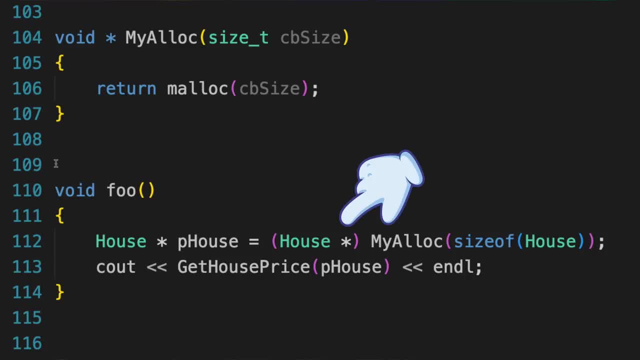 to cast that memory to almost any type they wish, such as a house object. Imagine that in our code we malloc and request enough bytes to hold a house. Malloc returns a void pointer which we immediately cast to be a house pointer. and now we can operate on that block of memory as though. 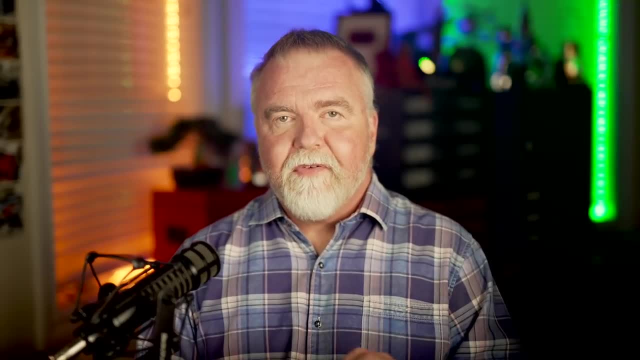 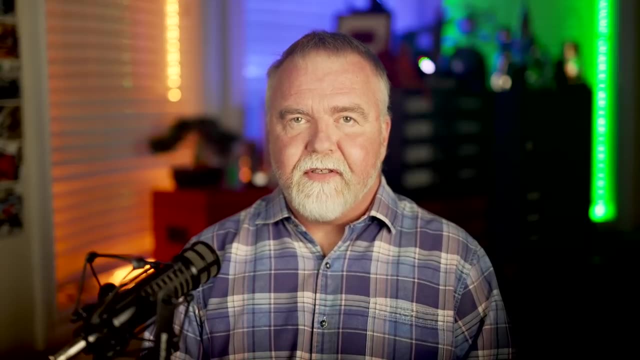 it has always been a house. Finally, we have function pointers, which are probably the most complicated form that you'll routinely run into. The function pointer does two things. Like any other pointer, it contains the address of something, which, in this case, is the address. 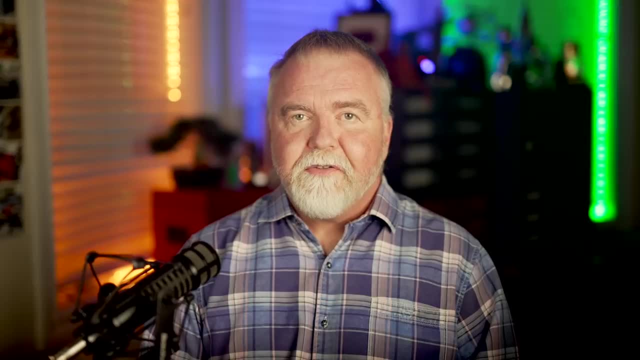 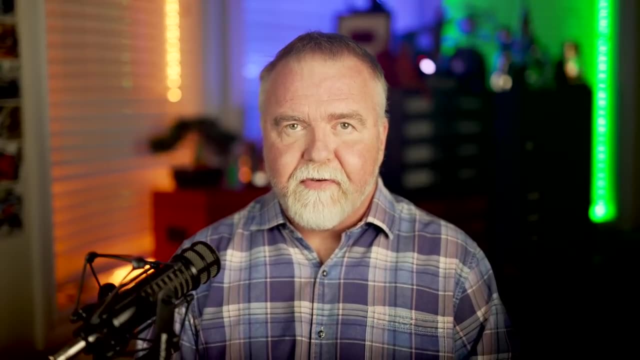 of a piece of code that implements a function. It also defines the arguments and return value to be expected when the function is called A function pointer, then is a pointer that points to a function instead of to a data type. This enables you to dynamically change which. 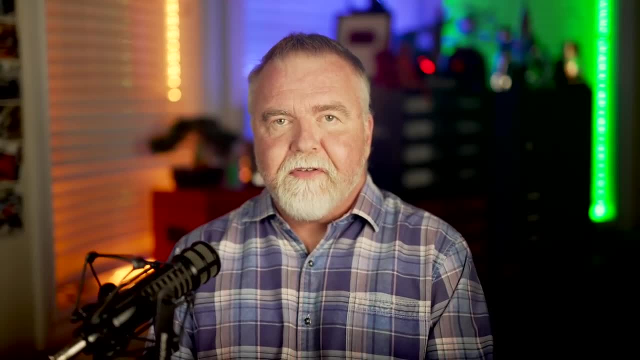 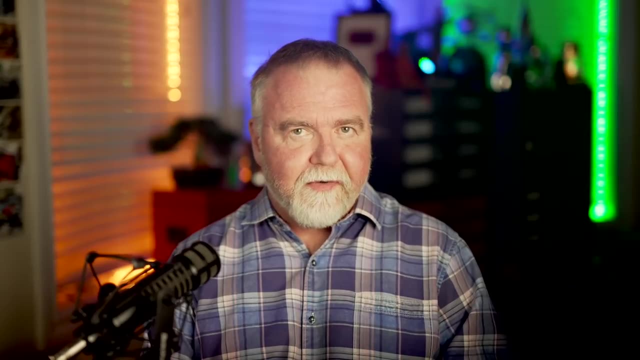 function is called in your program. You can think of function pointers as similar to normal pointers, but instead of referring to data values like an int or a char, they point to a piece of executable here. Here's how you can declare a function pointer. Here, pad is a pointer to a function. 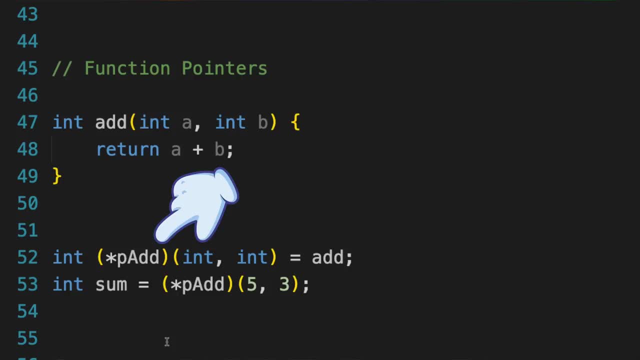 that takes two integers as arguments and returns an integer. The parentheses around star pad are necessary because of the operator precedence. Without them, the declaration would be parsed as a function declaration and not a function pointer. You can assign the address of the function add to the function pointer like this, and then you can use the function. 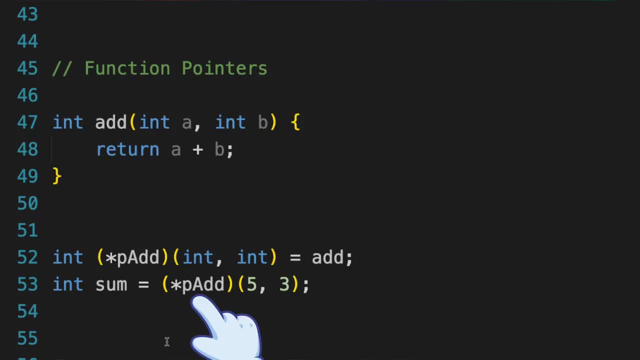 pointer to call the function. This will call the ADD function, with the arguments 5 and 3 and the. the result, which is 8, will be stored in the variable sum. Note that the parentheses around star p add are required when calling through the function pointer as well. Function pointers are: